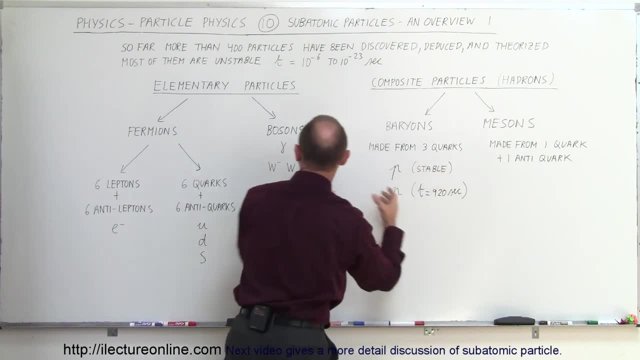 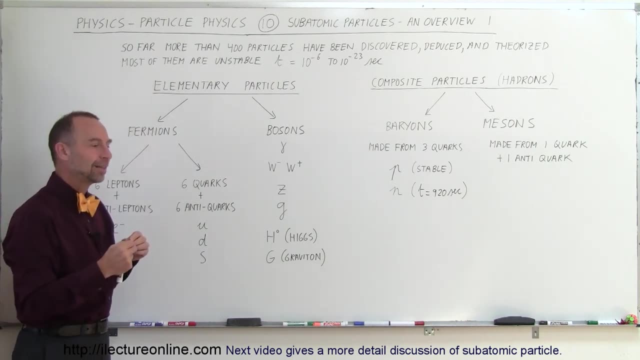 which are a conglomerate or a multiple set of the one or more of the elementary particles. Now, the elementary particles there's just one of those, So it's a unitary item, and of those elementary particles there are two different kinds. 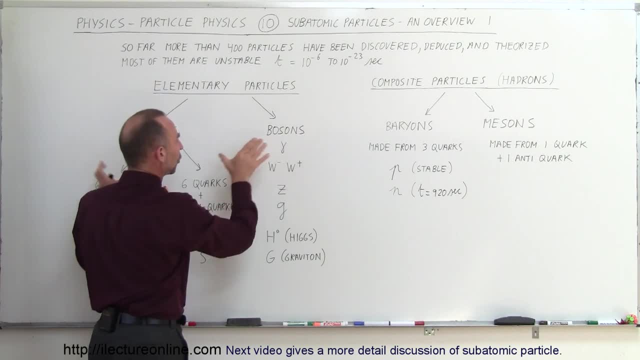 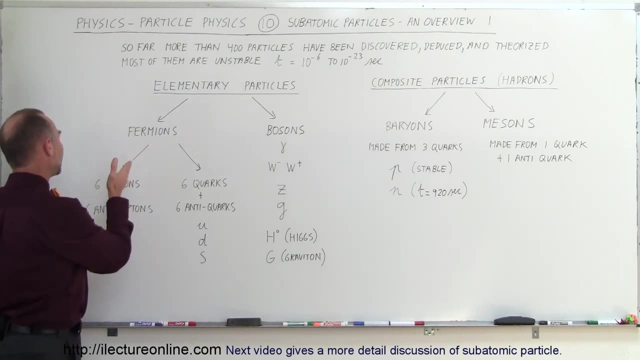 There's what we call fermions and there are bosons. So those are the basic elementary particles in the universe. Now, on the fermions, we have some that are called leptons and some that are called quarks. Now there's six leptons and then, of course, for every particle is an antiparticle. 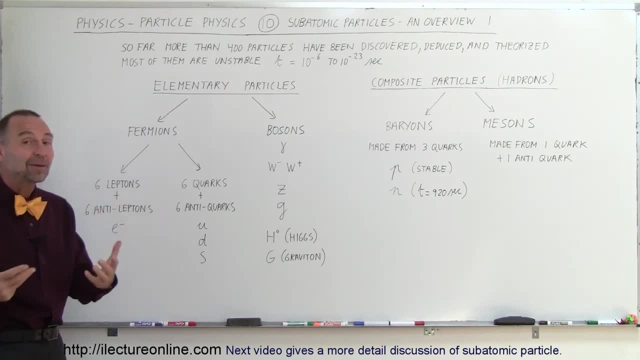 Therefore there must be six anti-leptons, And the most famous of those leptons is, of course, the electron. The electron falls in the classification of leptons, and there's five other particles that also fall in that classification. We'll show what they are later, in a different video. 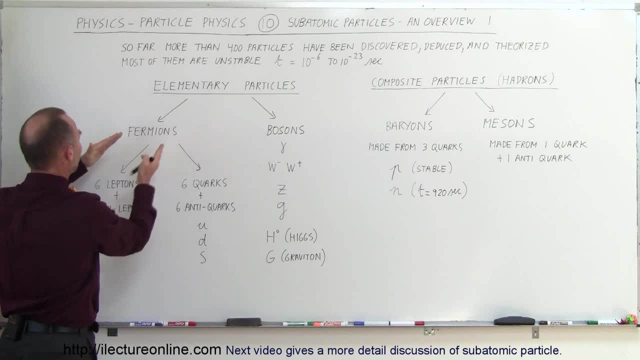 So, of the elementary particles, we have fermions. Of the fermions, we have leptons and quarks. Leptons are the very tiny point-like objects that don't seem to have any particular structure to them. There it is, They have mass, They have point-like existence. 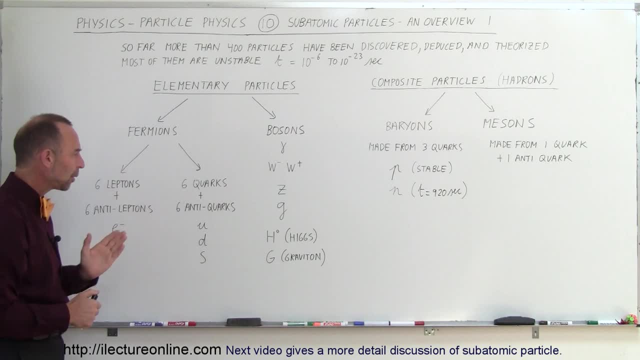 And there's six of those, electron being one of them. Then we have what we call quarks. Now, quarks have never been seen isolated by themselves, but they actually form objects that are bigger than the quarks, and they form what we call the composite particles. 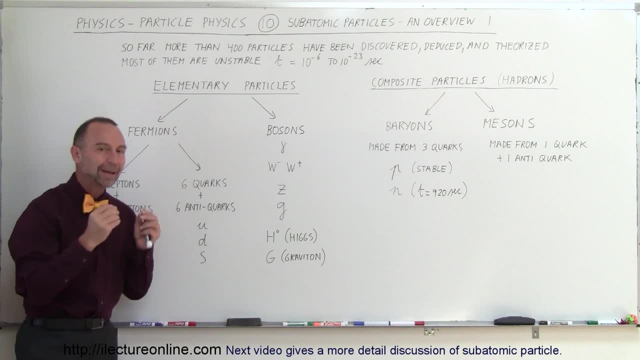 So the composite particles are made out of quarks. Quarks are the basic building blocks of the matter in the universe. The matter in the universe is primarily made of protons and neutrons, and so, therefore, the quarks are the basic building blocks of the protons and the neutrons. 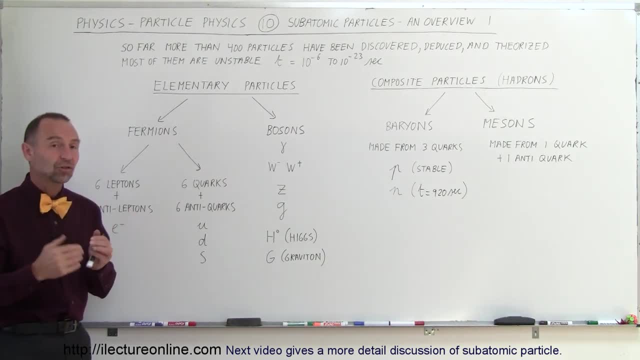 There are six different kinds of quarks and six anti-quarks associated with those six quarks. The three most famous quarks are the up quark, the down quark and the strange quark, The ones that are used to make. well, we don't make them, of course. 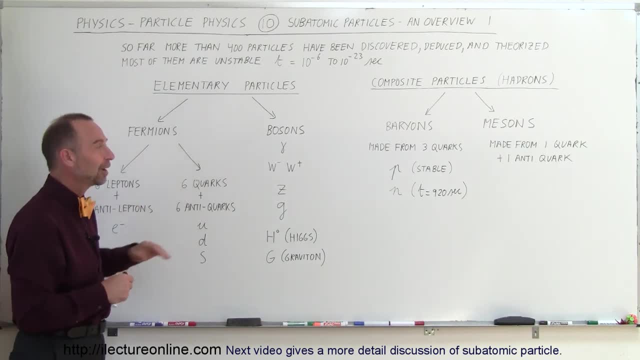 but up and down quarks in certain configurations will form the very famous particles- protons and neutrons- that everybody is familiar with, And we'll see later on how that happens. So there are six different quarks. The ones that make most of the particles that we're familiar with are the up the down and the strange quark. 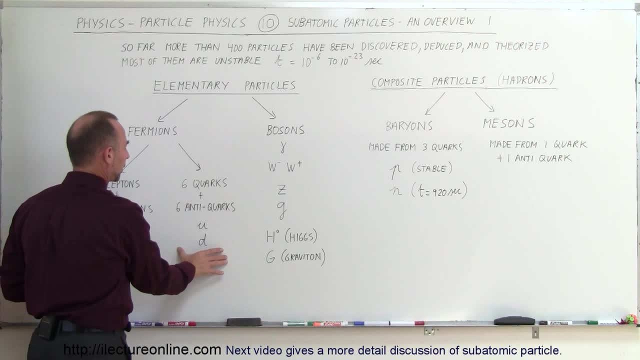 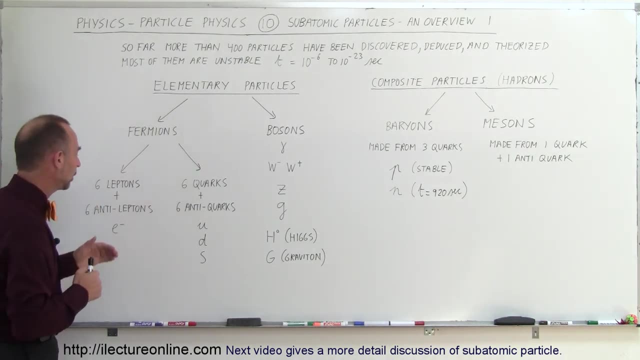 So those are the fermions that either make up the large particles that are conglomerates of the basic elementary particles, or we have the leptons, such as the electron that exists in unitary formation, And then we have what we call the bosons. 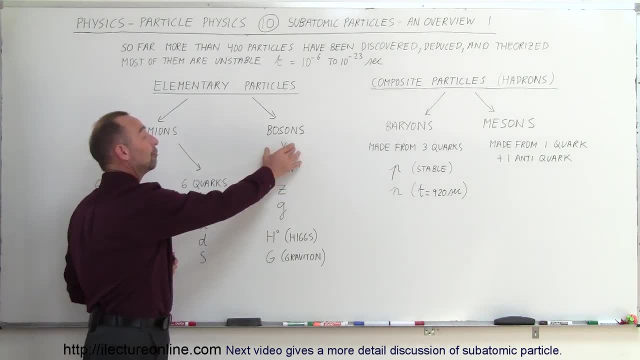 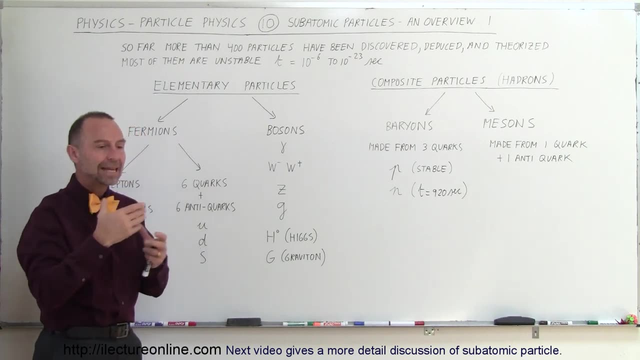 Now, the bosons are a very different kind of particle. It includes the photons, and the photons are just simply quantized chunks of energy and that is the mediating part of the electric field or of the electromagnetic force. We also have the W and the Z bosons. 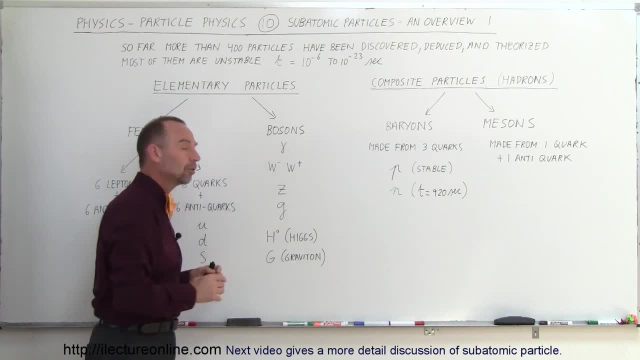 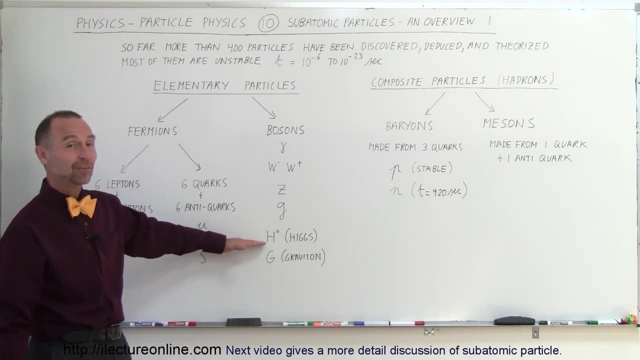 They also are intermediate particles. And then we have what we call the gluons. The gluons is what keeps the quarks together, But again, we'll talk about that later in more detail. And then, of course, we have the really famous particle that was discovered in 2012. 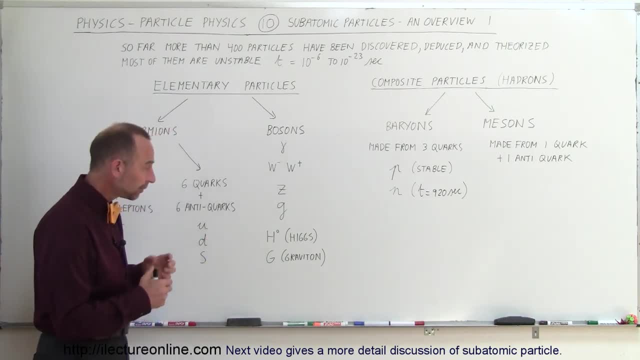 in CERN, at the very large accelerator, And we believe that the Higgs boson is responsible for causing the Higgs field which gives the particles mass, And so we'll get into that a little bit later. And of course we have the elusive graviton, which we haven't found yet. 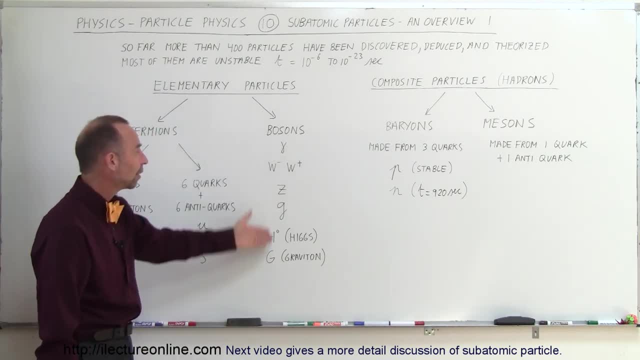 but we feel there probably is such a thing, And so that would then be part of what we call the boson particles or bosons. And so those are again the elementary particles. They cannot be broken down or subdivided, And that is the key difference between elementary particles and composite particles. 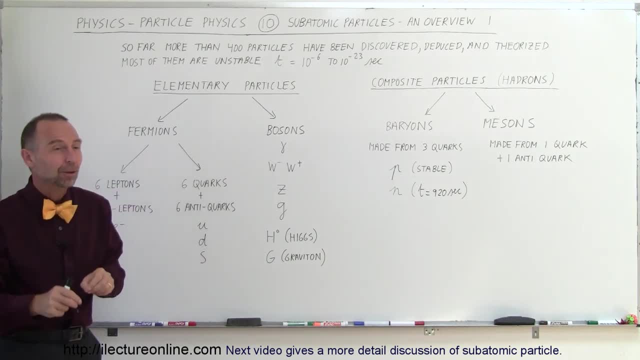 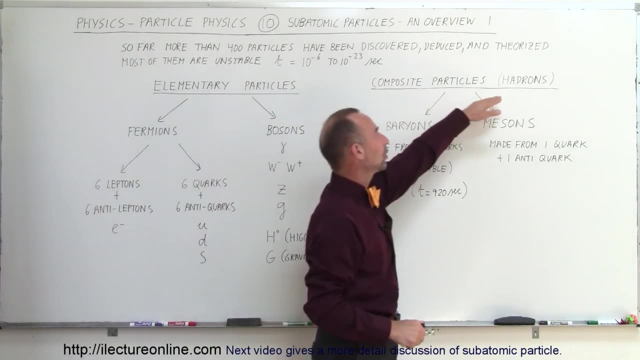 that these particles cannot be broken down any further into smaller particles, at least not that we know of at this point. And the composite particles are called hadrons. Hadrons means heavy particles, They're much bigger. And of those things, of the composite particles, 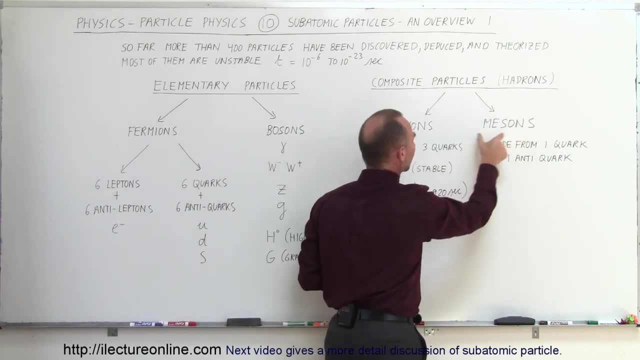 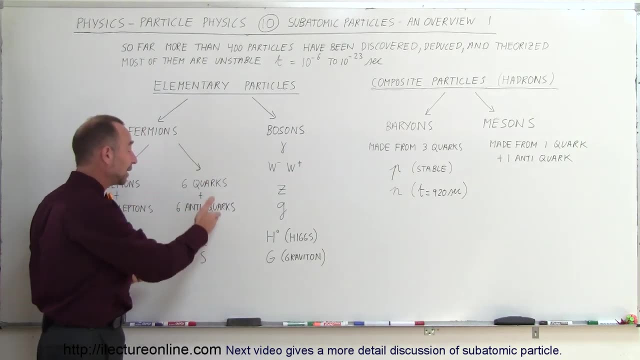 there's two main types: There's the baryons and there are the mesons. Now the baryons: they're made from three quarks, So a combination of these three quarks, and there's baryons that are also made from the other three quarks. 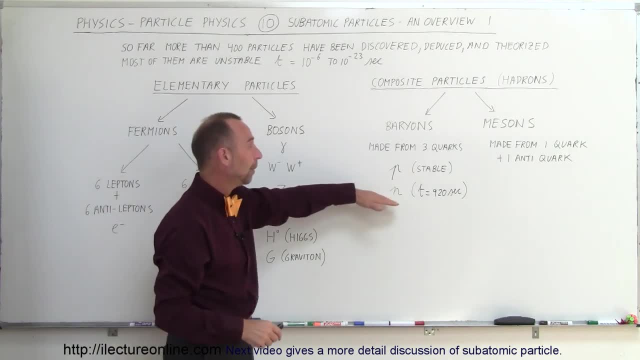 that we haven't talked about yet. But the most stable particle, well, the one that is the only one that is really stable of the composite particles, is the proton. The proton by itself is very stable. That is the end product of any other, what we call baryon. 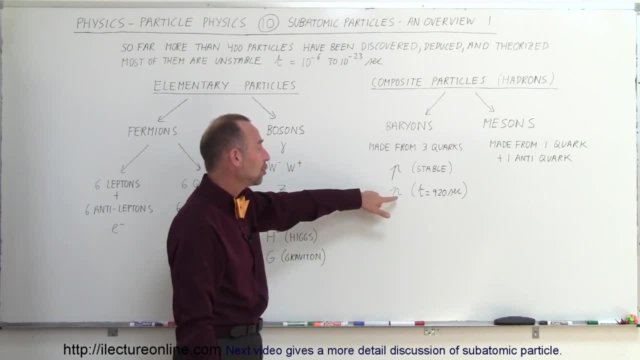 that will disintegrate into a different particle. And then we have the neutrons. Now you would say, well, wait a minute. Isn't all matter made of protons and neutrons, and therefore shouldn't the neutrons be stable? 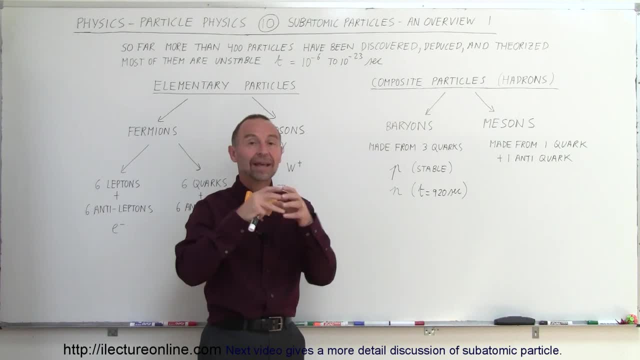 And it turns out a neutron positioned inside a nucleus tends to be stable, But a neutron inside or not inside a nucleus, but by itself, tends to be very unstable. It has a typical lifespan of about 920 seconds before it disintegrates. 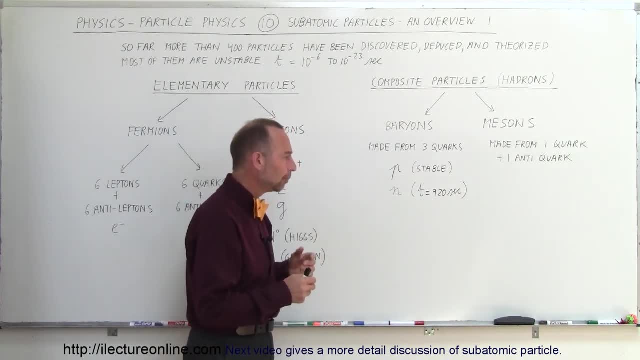 That's kind of like the half-life of a neutron, But inside a nucleus they tend to be more stable. However, in nuclear decay it's usually the neutron that changes into a proton, into something else, So there's a decay process that's associated with the neutron as well. 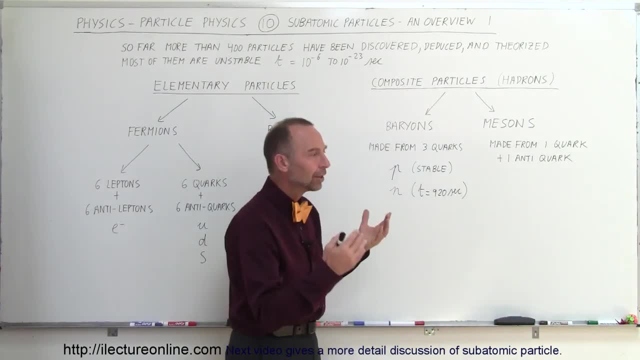 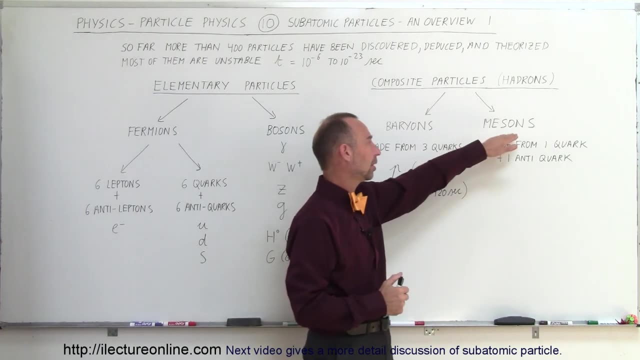 Now the mesons. those are what we call the middle particles, as we call them, because they're not as heavy as protons, but heavier than electrons. They fall somewhere in between. That's why they're called mesons. They're made up of one quark and one anti-quark. 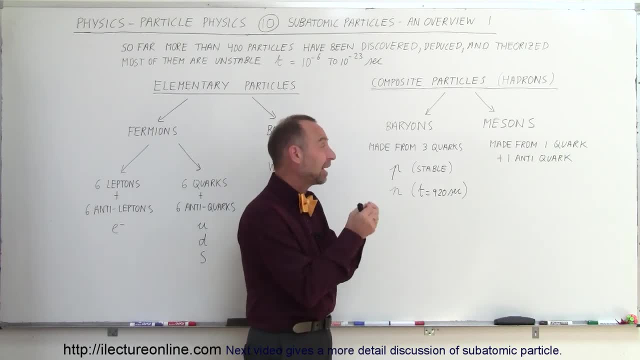 That makes them very unstable and they only typically last a very short amount of time. So we'll find out later that all of the mesons are very unstable, only stick around for a very short period of time. The baryons are all very unstable. 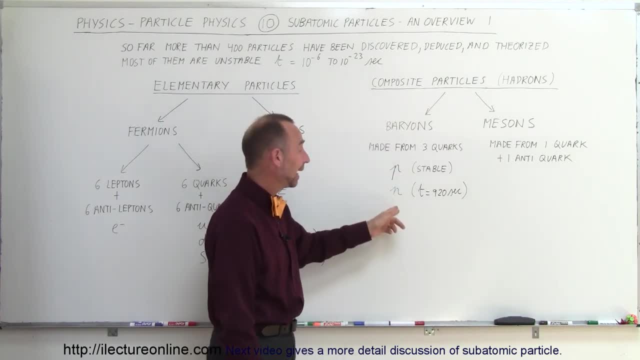 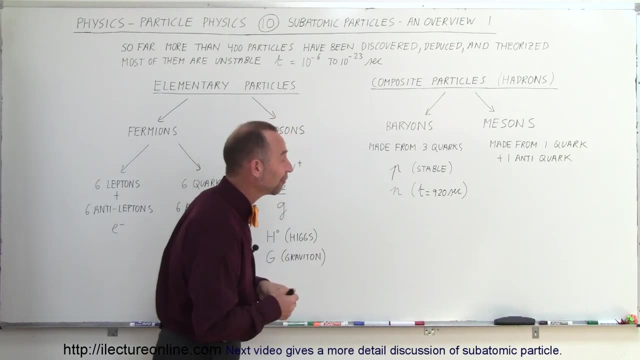 except for the proton, which is very stable, and the neutron, which is only stable inside the nucleus and not so bad, lasts under 20 seconds when it's a free neutron, as we call it. So this gives you a very general picture. 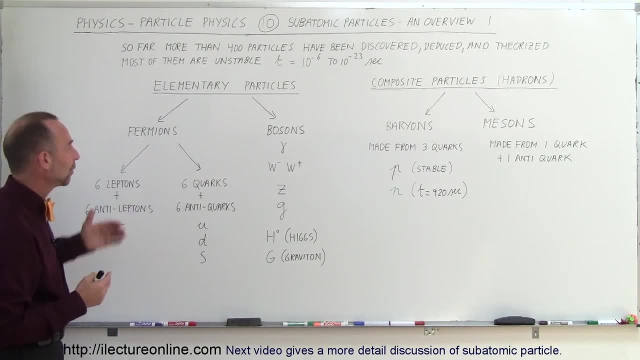 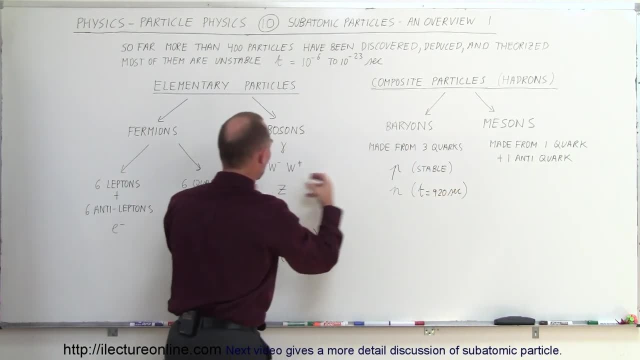 of the way subatomic particles are laid out. So we have the elementary particles, which are like point-like objects that cannot be subdivided. We have the composite particles, which are all made out of quarks, so some sort of combination of quarks. 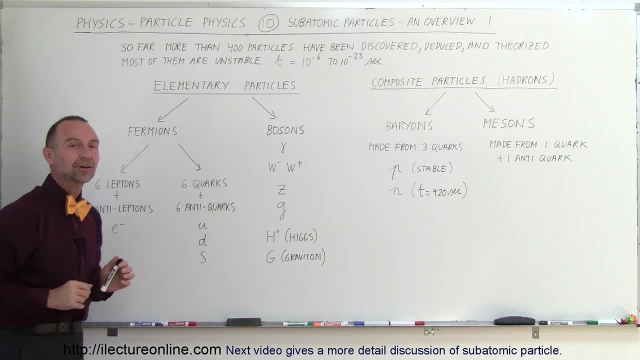 So it looks like quarks are the basic building blocks of matter in the universe. Fermions are used within the building blocks to be able to form atoms and things like that, And some of the fermions, or leptons and anti-leptons. 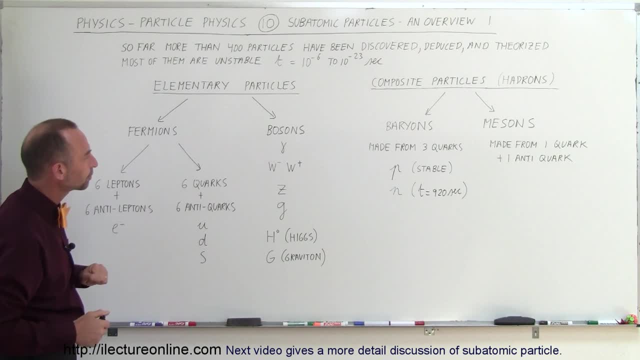 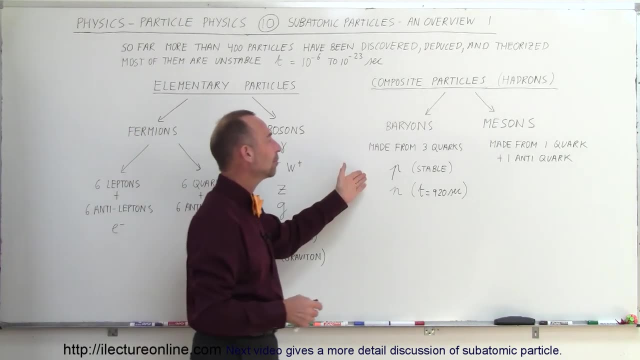 are also a byproduct of certain nuclear processes. Bosons tend to be the interaction particles, the mediating particles for the four forces in the universe, And the composite particles are conglomerates of quarks which are used to make up matter in the universe.